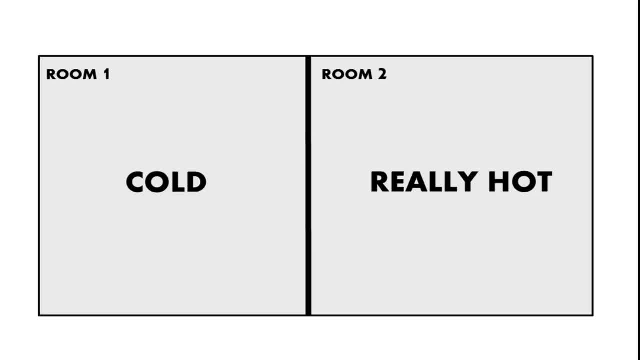 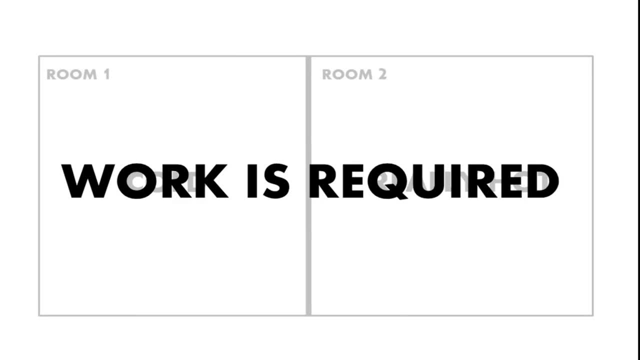 room one cold and room two really hot. How could we do this? Well, the second law of thermodynamics says that work is required, but if we are willing to put in the work, it is possible. So how could we create something to actually pump heat from room one into room two? Well, 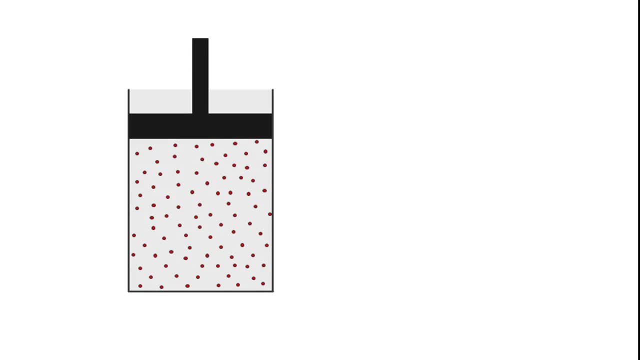 we are going to use this principle of thermal character And I'm going to be using Koller wr statistical of compressing and decompressing gases. So if we have a piston filled with gas and we compress it, it will heat up. Then if we allow that heat to escape and release our hand, 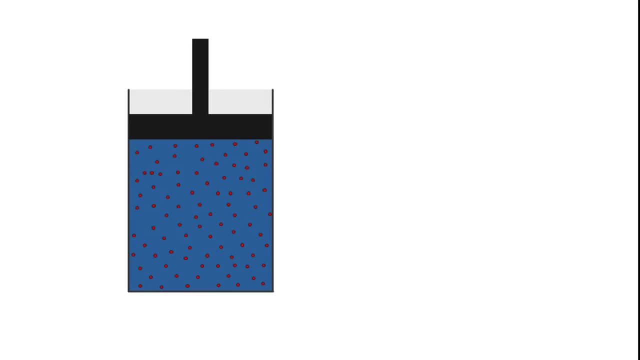 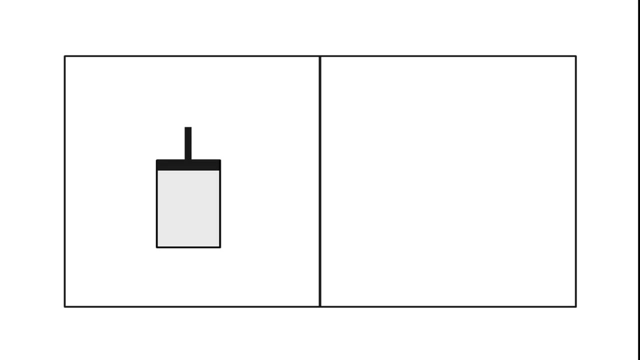 the gas will expand, decreasing its internal energy and cooling down. It's this principle that we're gonna use to build our refrigeration device. So here we have room one and room two and we have a container filled with gas, which I will just call a refrigerant. 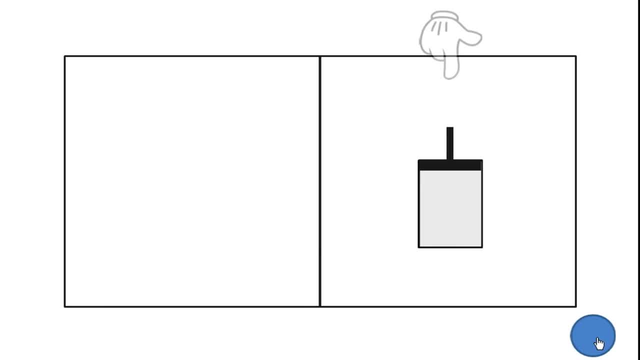 Now this is how it works. If we move the container to room two, compress it so it heats up and allow that heat to escape, and then move the container back to room one and allow it to decompress, then the heat from room one will move into the container. 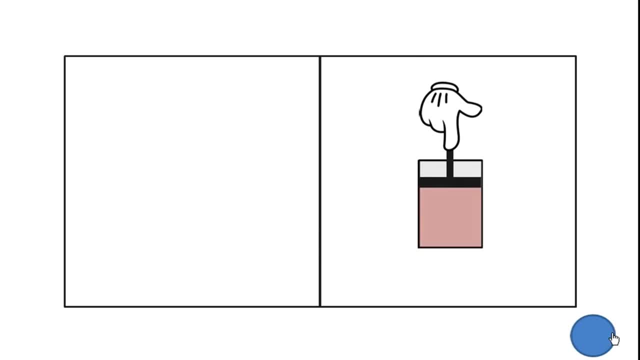 If we repeated this process over and over and over again, eventually the heat from room one will be pumped to room two. Now, if we look at all of the components into making this happen, we see that there are only really three essential pieces. The first piece is some sort of transport medium. 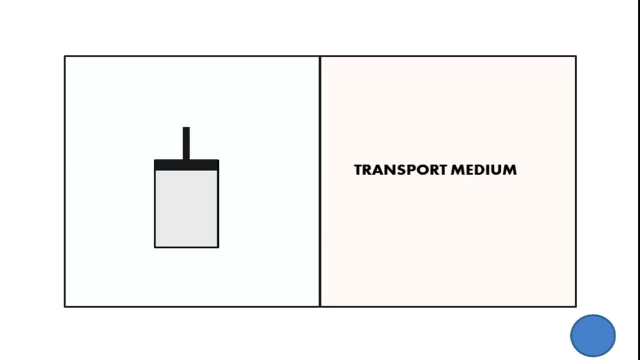 So this is the container that is filled with the gas or the refrigerant. The second important component is some compressor, In this example, that hand that compresses. the piston plays the role of the compressor, And the third important component is the decompressor. 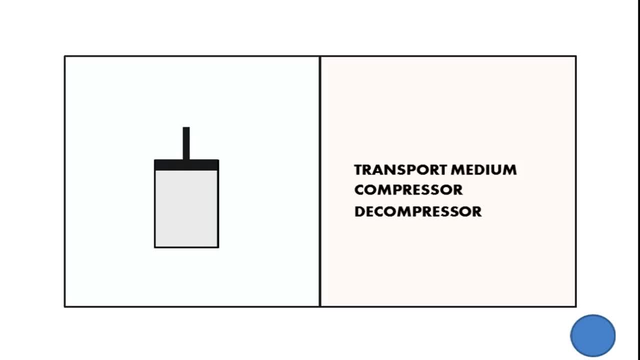 In this case we have a piston that as the gas expands, it lifts up that piston. If we have these three components, we can build some sort of device. We can build some sort of device. We can build some sort of device that transports heat from one room to the other. 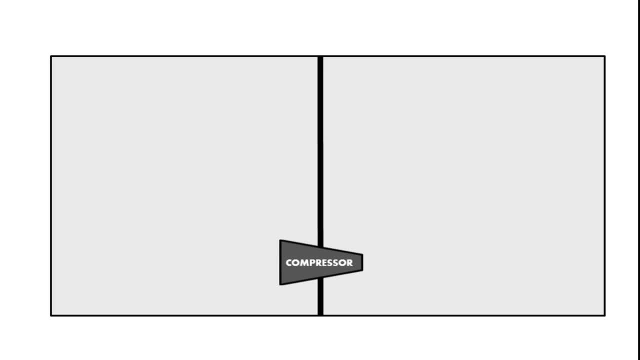 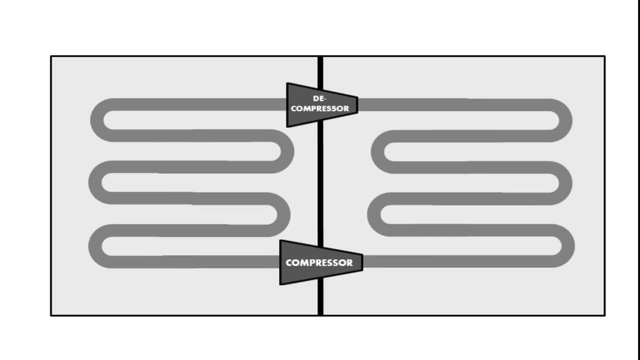 Now we have two rooms and we build in a compressor that simply plays the role of compressing gases. We also build in a decompressor that does the very same thing, except the opposite, If we connect both of these rooms to a set of tubes carrying some sort of refrigerant like a gas. 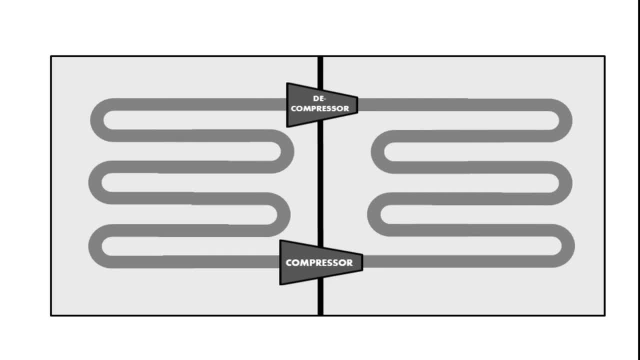 or a liquid that becomes a gas, then we have all three necessary components. As this gas is pumped through the compressor, it will heat up, and as it heats up, that hot gas will travel through these long S curves and cool down over time. 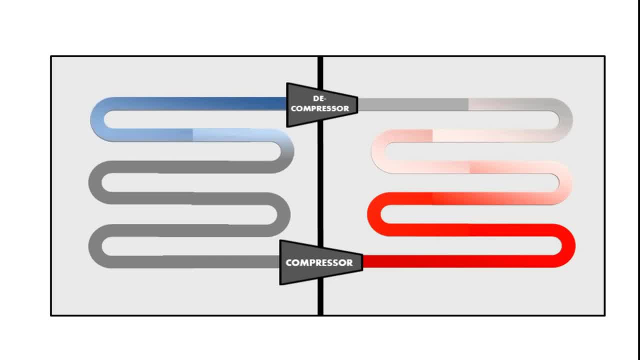 And when the gas goes through the decompressor it's gonna rapidly cool down. So on the other side of the decompressor we have this very cold gas that slowly warms up as it goes around the curves. So you can imagine this gas being pumped through these wires. 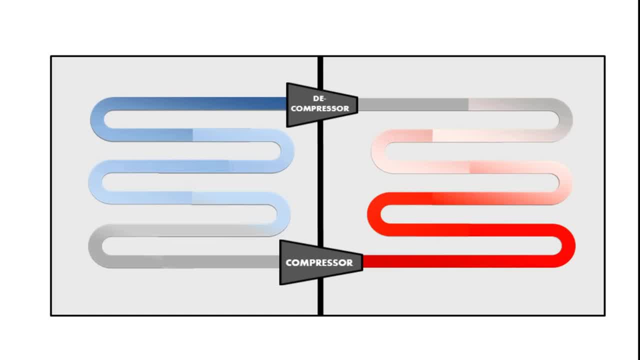 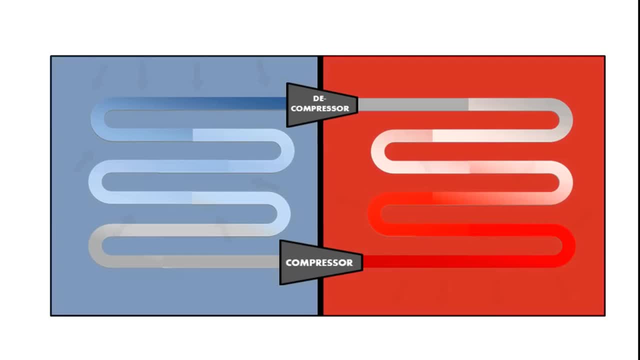 through the compressor than the decompressor. again and again, and again, And eventually heat is gonna be pumped from this room over to the second room. So we're gonna find one room that gets really cold and then the other room that gets really hot, And this is exactly how a refrigerator works. 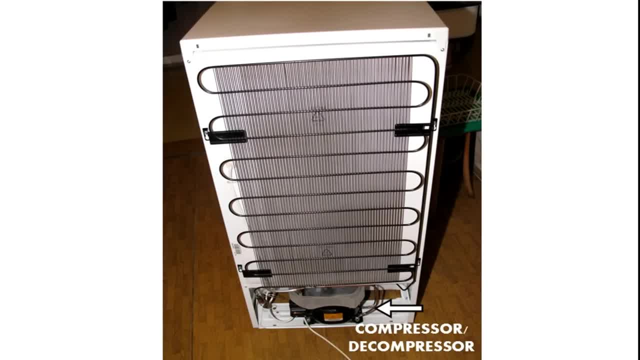 So here is the back of a refrigerator. Right here we see this motor that plays both the role of the compressor and the decompressor, And then we see the cooling coils on one side of the refrigerator. Inside is an identical set of cooling coils. 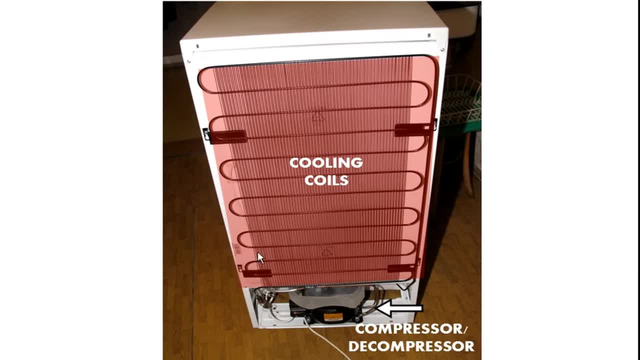 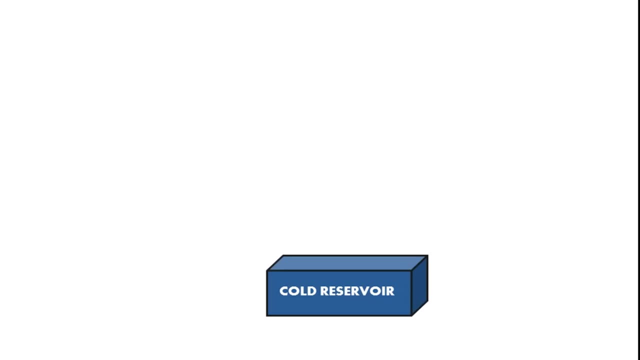 So hot compressed gas moves through these outer coils and cools down, and then it hits the decompressor and cold gas flows through the inside, cooling everything on the inside of the refrigerator down. Now if we build a diagram of a refrigeration unit, it would take something from a cold reservoir. 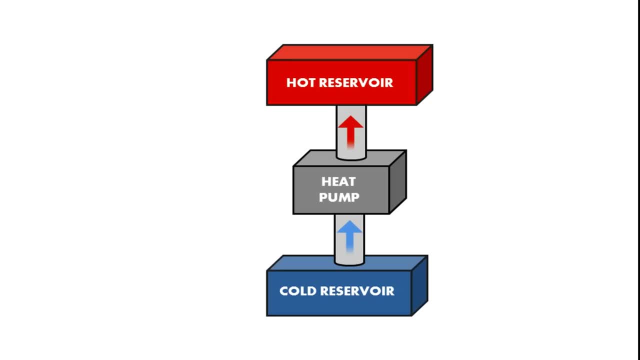 and pump heat from the cold reservoir to the hot reservoir. But the second law of thermodynamics says that this process does not happen spontaneously. It takes a certain amount of heat and then put a certain amount of work, So the work that goes in actually produces heat. 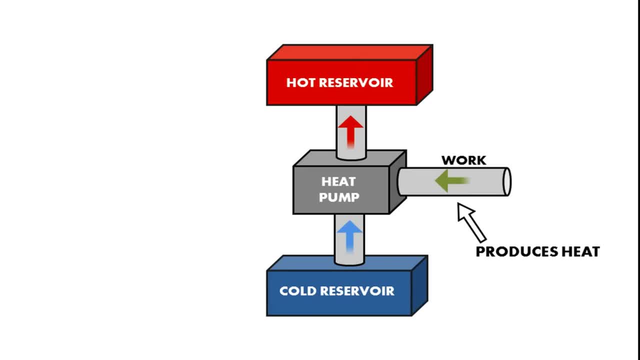 This means that the heat that comes out of the cold reservoir does not equal the amount of heat going into the hot reservoir. But we see that there's more heat going into the hot reservoir than coming out of the cold reservoir. The process of pumping heat from one place to another. 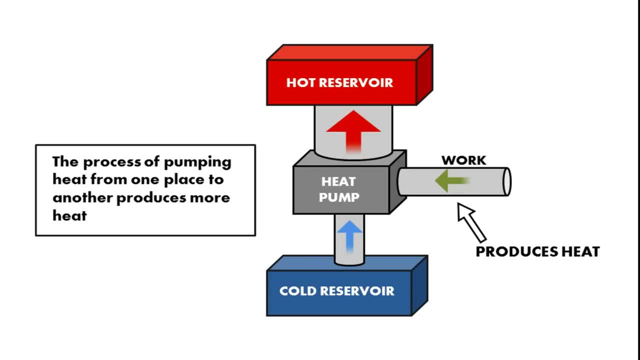 produces more heat. Now, this is good news and bad news. The bad news is this means you can't really cool your room down using a refrigerator. If you open a refrigerator door, then you're going to draw in heat from the outside. And as more heat is drawn from the outside, 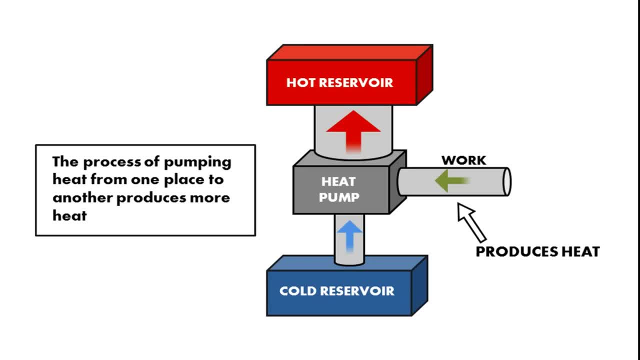 you're going to kick on that pump which produces more heat, And that heat is dumped back to the outside world. This means, if you don't close your refrigerator door, eventually the refrigerator will make your room much hotter than it would have been had you just kept it closed to begin with. 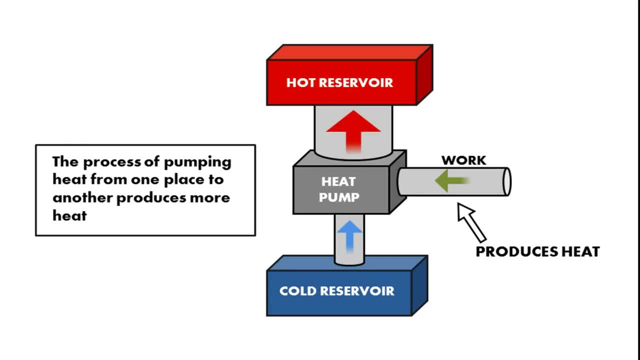 The good news is we can design some sort of heat pump that takes heat in from the cold, from the cold outside, and pumps it into the inside on days when it's kind of cold. So imagine now we compare these two different types of heaters. 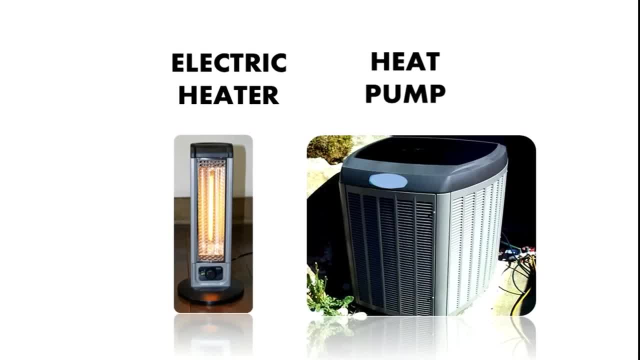 an electric heater and a heat pump. On the right is a heat pump and on the left is an electric heater. Now, an electric heater works by warming up wires, by passing electrons through these wires. Heat pumps work on the process of reverse refrigeration. 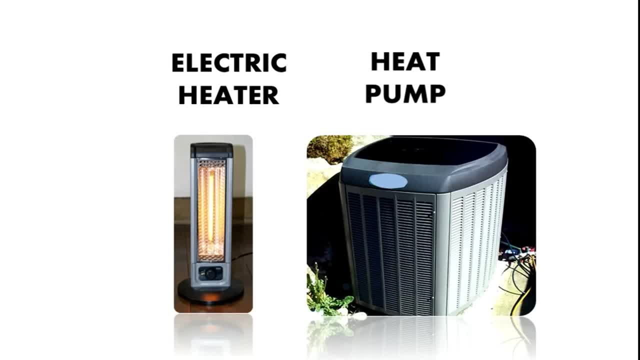 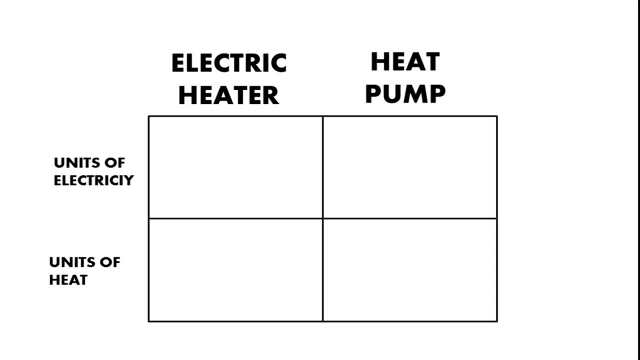 They pump heat from the cold outside into the warm inside. Now if we were to compare the amount of electrical units it takes to run an electric heater and the amount of heat each one of these heaters produces, we will find something very interesting. An electric heater may take plus one units of energy to run. 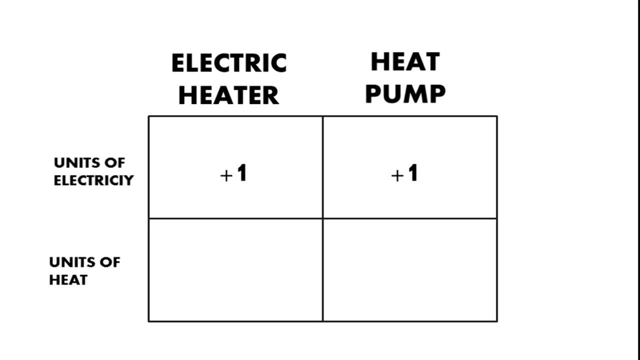 Likewise, a heat pump may take plus one units, But the heat that we get out of an electric heater can only get to plus one units of heat. This is because energy is conserved. The amount of energy that goes into the electric heater must be equal to the amount of energy that comes out. 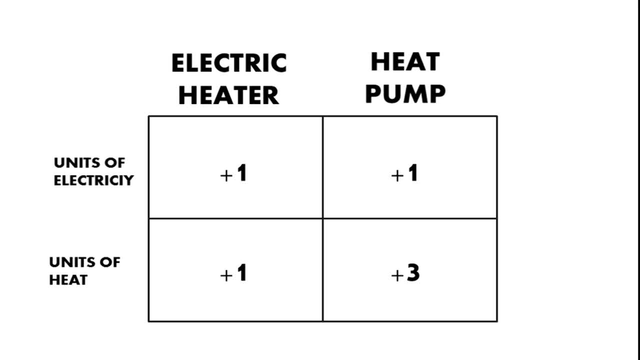 But the heat pump works by different principles. It can actually get more heat out than electric energy is put in. How is this possible? Is this a violation of the conservation of energy? Well, actually no, Because the heat that comes out of the heat pump. 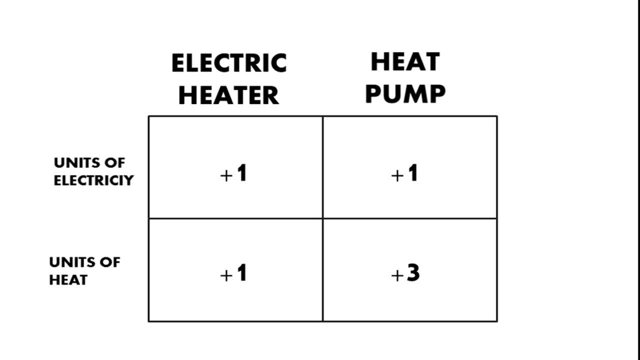 comes from outside, So we get a bonus. We get heat that's drawn in from cold air and we get the bonus heat that's produced in the process of making this happen. So we find that heat pumps are much more efficient at producing heat than an electric heater. 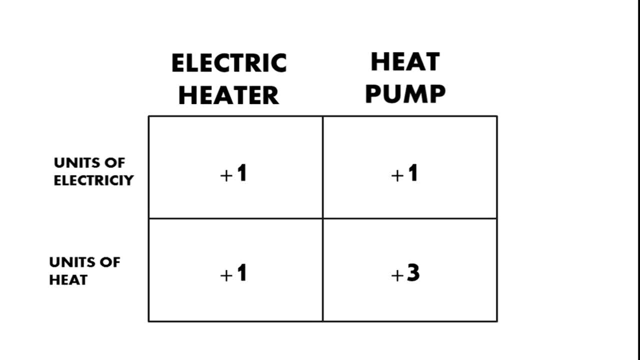 And something that should always be considered when designing an energy efficient home.